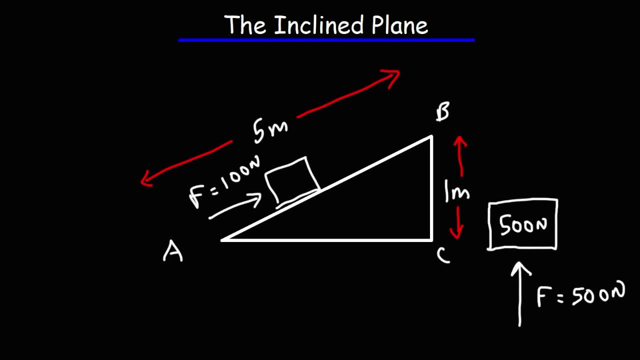 500 newtons of force, we can go from A to B, which will require less effort, or 100 newtons of force, And so the incline plane makes it easier to move heavy objects from one place to another, Especially if you need to go up. However, there is a cost, though This doesn't come free. 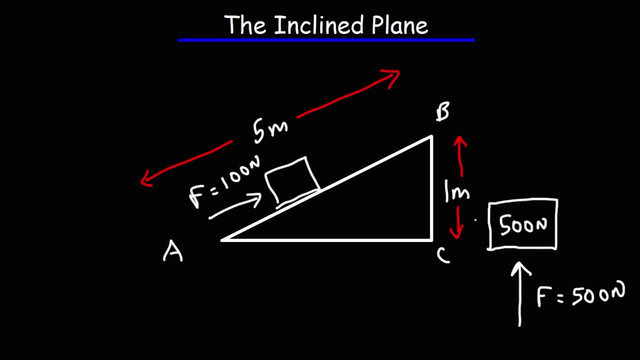 And the cost is the distance to go from C to B. It's true that we need to apply a greater force, but only over a shorter distance. So if we were to calculate, work is force times distance, that's 500 newtons times one meter, so that's a work of 500 joules. 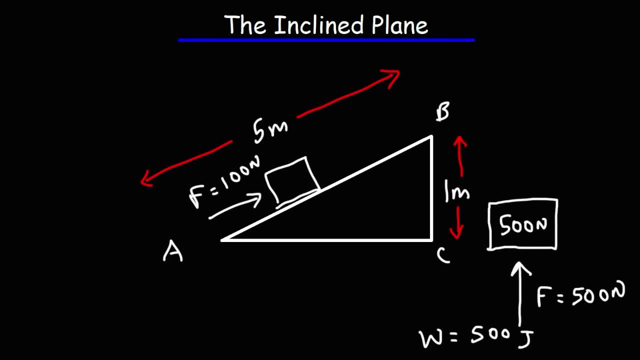 now we can go to from a to b, which requires less effort, but i mean we're going for a longer distance. if we calculate the work going from a to b, that's 100 newtons times five meters, which is also 500 joules. so the simple machine doesn't really reduce the amount of work that we 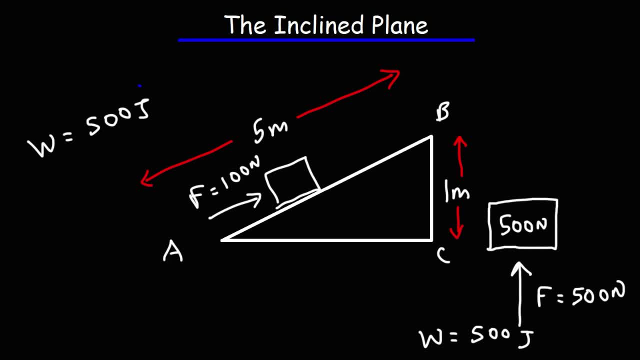 need to do. the work is still the same. regardless of what path we take- a to b or c to b- the work doesn't change. however, the effort that's required does change. it's harder to go from c to b because we need to apply more force, even though it's for shorter duration, but going from a to b we can. 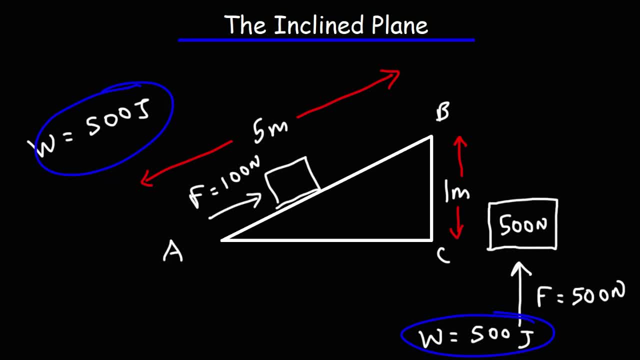 apply more force and we can apply more force to the work that we need to do. so we can apply more, less force, but for a longer distance. so the inclined plane makes it easier to get the work done, but it doesn't change the amount of work that needs to be done, and it's important to 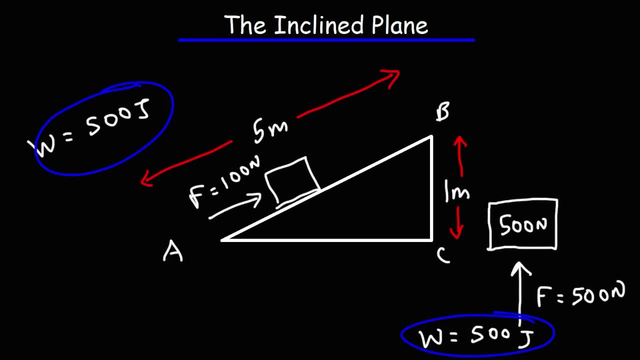 understand that concept. now, the situation that we're dealing with here is a frictionless inclined plane, so this is an ideal scenario, but in reality, whenever you're moving an object across the surface, you need to deal with friction. there's always going to be some amount of friction present, which can vary based on the two types of services, and so the amount 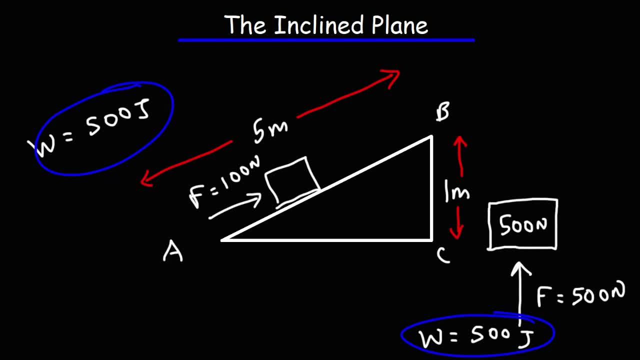 of force that you're going to need to move it up, the ramp is going to be more than 100. in reality, it could be 120, it could be 130, it could be 140. it's not going to be as high as 500, but because of friction it's going to be more than 100. and just as you can't make money without 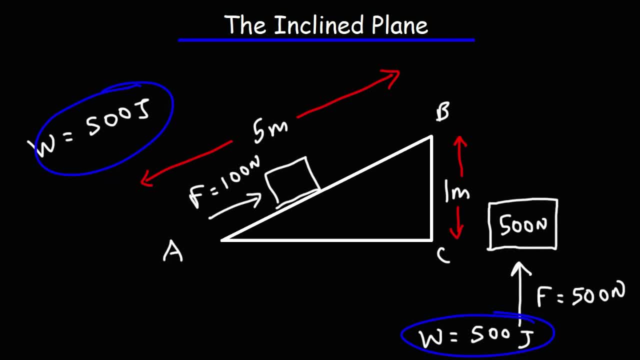 paying taxes. at least you really shouldn't. you have to pay your taxes. you can't really do work without paying energy to friction. anytime you do some type of work or exert some type of force, especially across the surface, some of the energy that you're applying to get the work done is going to be spent on friction or dissipated as heat in some instance. 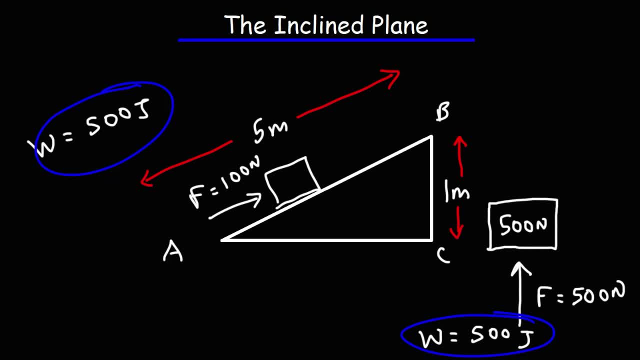 and that's just a fact of life. friction and dissipated heat is basically the tax in the energy world. you can't escape that, but nevertheless, the incline plane is a very useful machine that can reduce the amount of effort that's required to do some type of work now. another thing we need to talk about is 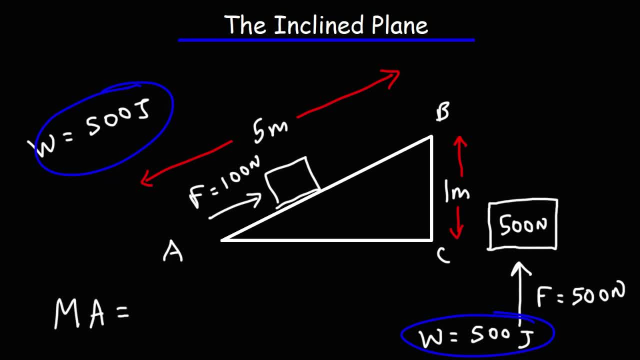 something called mechanical advantage. the mechanical advantage basically tells us the amount of force that- or rather the ratio of the two forces that the machine really assists in with. so it requires 500 newtons of force to go from C to B, but we're only using 100 newtons of. 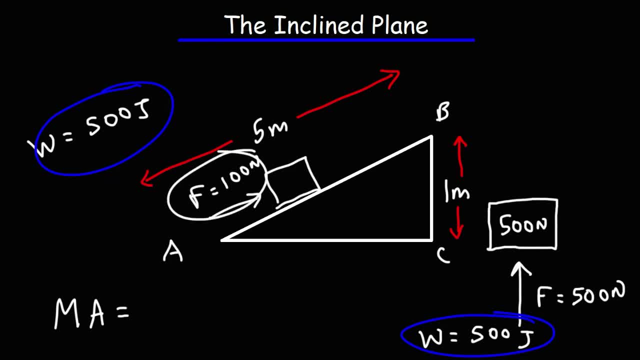 force to go from A to B. so you could think of this as the input force and as the output force. so this machine made our effort five times less, so we can say that it's mechanical advantage is five. our effort has been reduced by a factor of five. 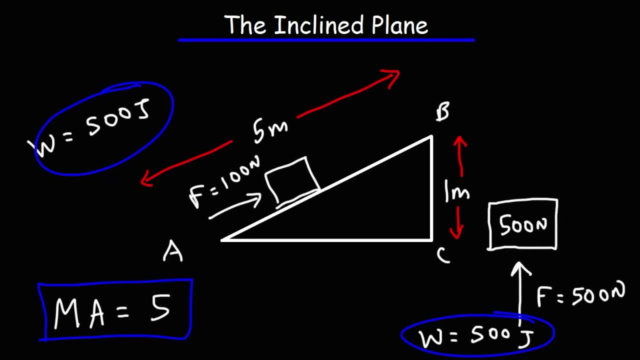 so that's the mechanical vantage of this particular incline. it's the ratio of the two forces. if the mechanical advantage is less than one, then you're applying more force than the machine is putting out. but if the mechanical advantage is greater than one, like five, then the machine is making your work five times. 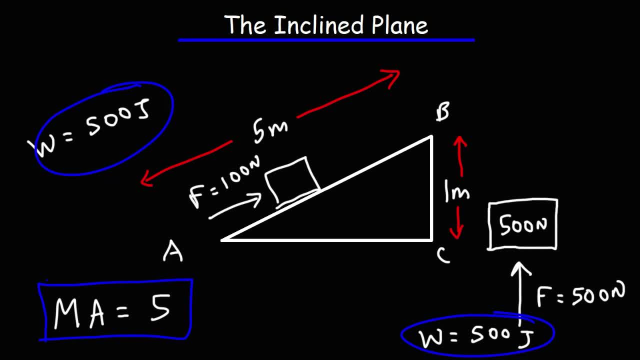 easier. it's multiplying the force by a factor of five. so even though you're applying a force of a hundred, it would've been equivalent to a applying a force of 500 going up. So it's making the work five times easier. So that's the basics of the incline plane. 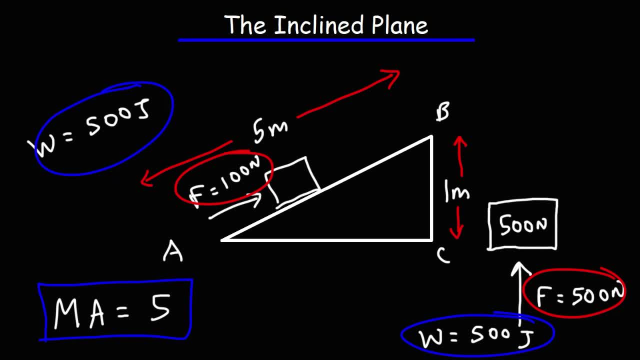 That's how it works. So now you know how to calculate the mechanical advantage and the force that's required to go up the ramp without taking friction into account. So that's it for this video. Hopefully you found it to be educational. Thanks for watching.